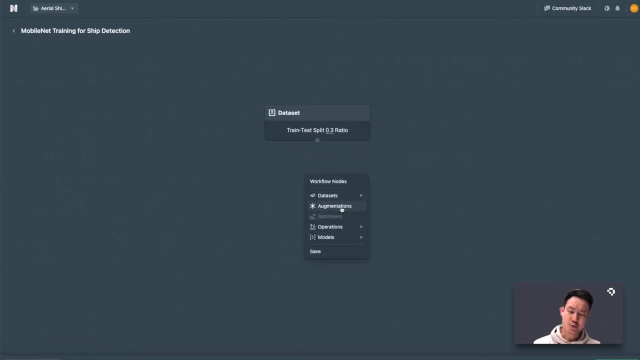 So first we can drop a dataset node, connect it to augmentations to create some augmentations for our training, to improve the robustness of the results. We can also perhaps add image scaling And finally let's add the MobileNet model. 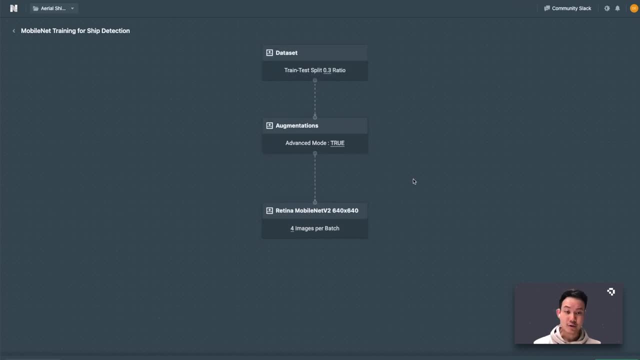 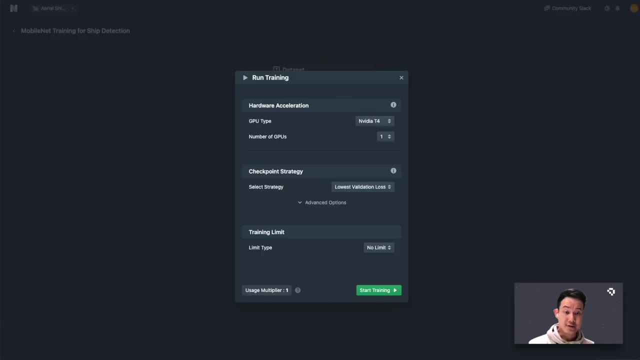 So this visual workflow will instruct Datashare to create this particular workflow in TensorFlow on our servers. For this training, let's use a 5,000 view March. The Datashare platform also supports multi-GPU training, But since we are just training a, 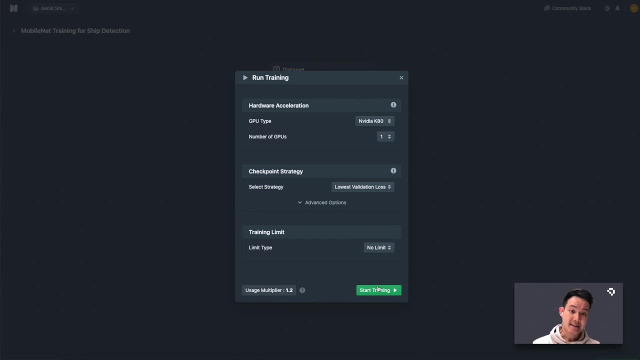 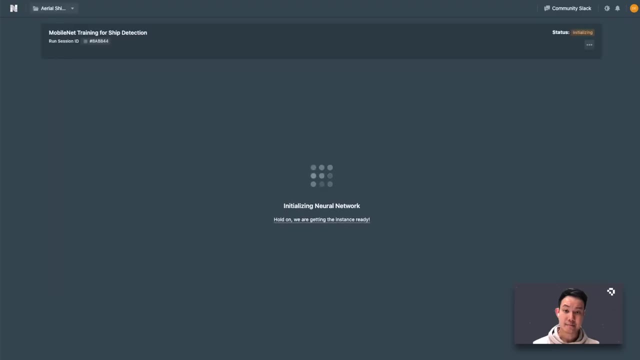 MobileNet, let's just use a single KAD And let's select the lowest validation loss as our checkpoint strategy to identify the best widths or checkpoints to use. at the end of the experiment, The server takes 2-3 minutes to set this up as it's preprocessing the images. 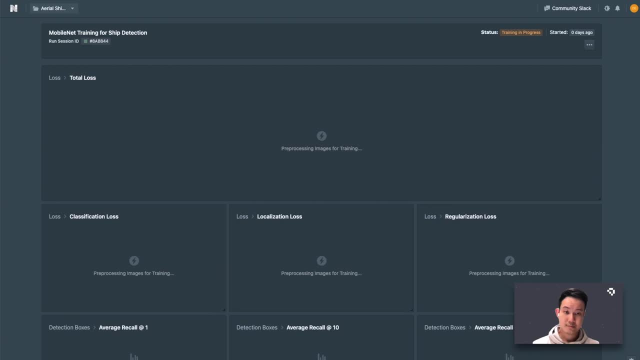 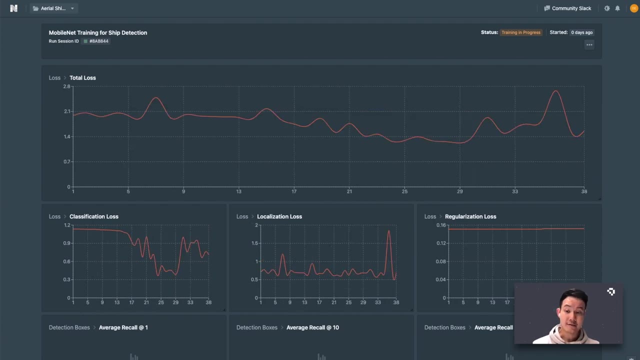 ready, the developer and team will be greeted with a real-time metric monitoring of the 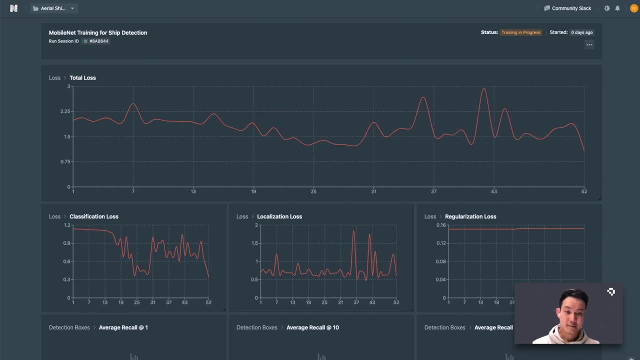 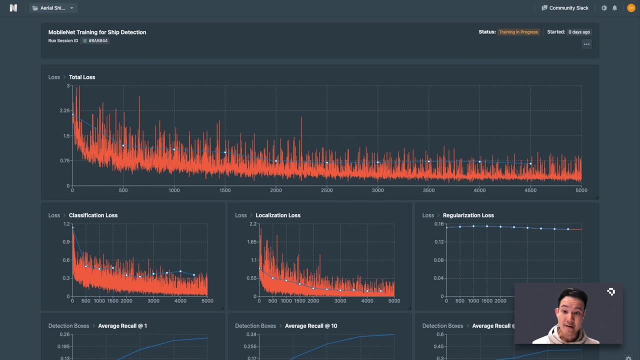 model training. Since this is a mobile net of 5,000 imports, it should take roughly about an hour to complete its training. And there we have it. We see a blue line which indicates the evaluation values of this particular training And, looking closely, we see that the checkpoint at 4,500 yields the least loss. 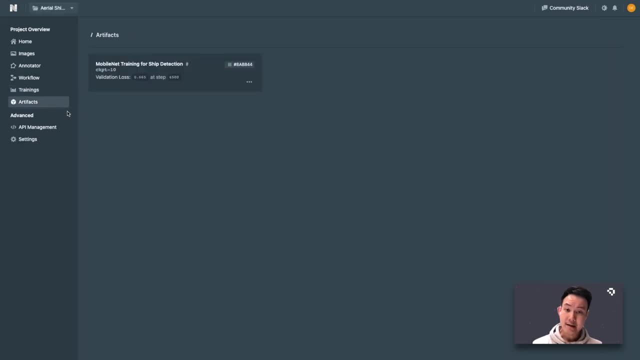 So let's use that for our experiment. We see that the training pipeline has already prepared this in artifacts, since we selected the lowest validation loss earlier, So let's generate a TensorFlow model so that we can use it in our own project. This model can be deployed on mobile phones, IoT devices and much more. 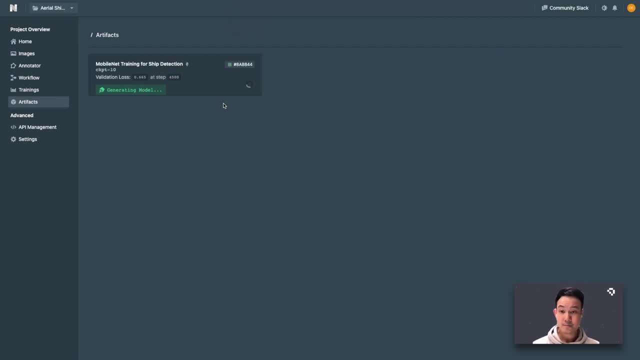 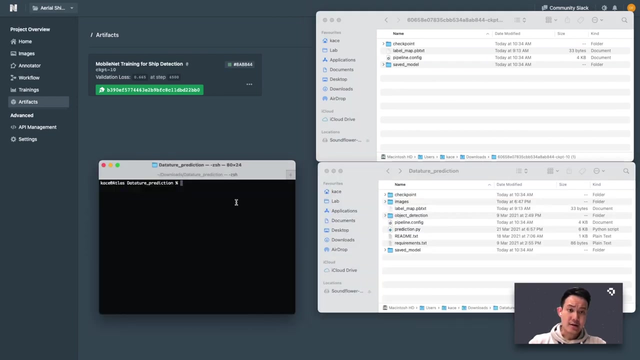 But in this case let's run it off my computer And it's ready, So let's download it and import it to our project. We see the folder showing the content of the downloaded file. Let's track the model and its weights into our project folder. 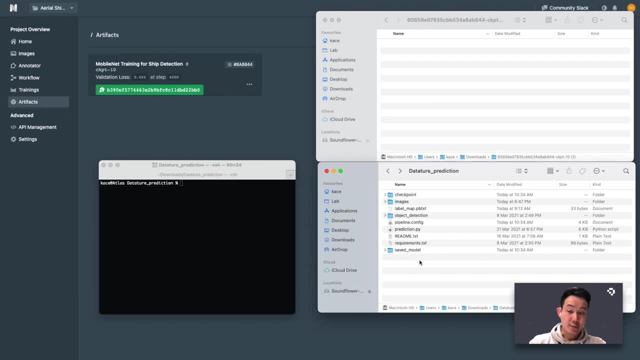 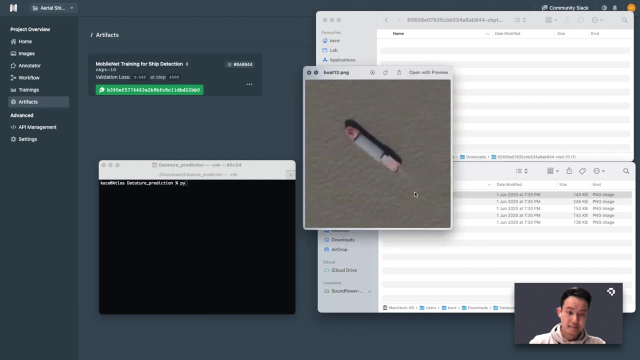 I have prepared some validation images so that we can test this model and its efficacy. Let's create an output folder so that we can save our prediction or inference results. Cool, Let's do this. Yay, Yay, Yay Yay.